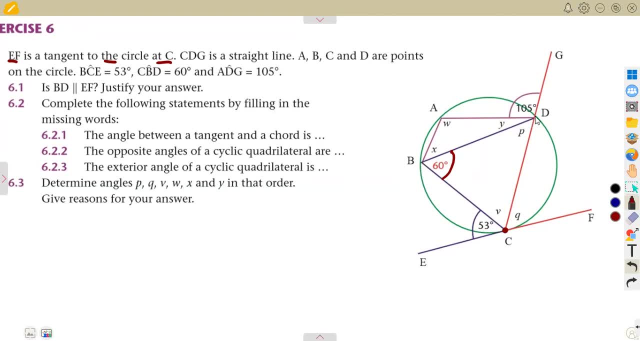 And also A D G. from A to D to G is 105.. We are also indicated there, 6.1, is B D parallel to EF? Justify your, it's a question. It's a question They are asking you: are these two lines parallel, Line B D and the line EF? are they parallel? 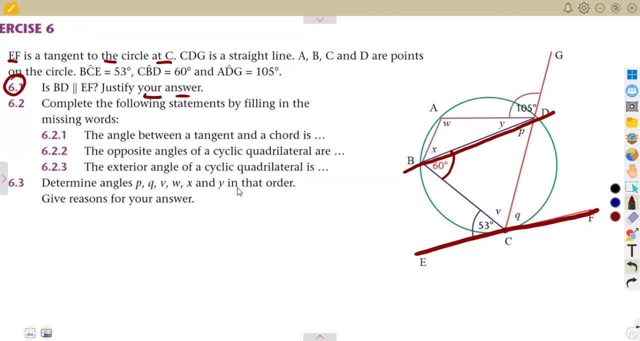 If they are parallel, meaning to say we must or we are supposed to have anything, any theorem about it. If they are parallel, meaning to say we must or we are supposed to have anything any theorem about it, They are supposed to be equal. But these angles, they are not equal. This angle that we are seeing here is 60.. This angle is 53 degrees. 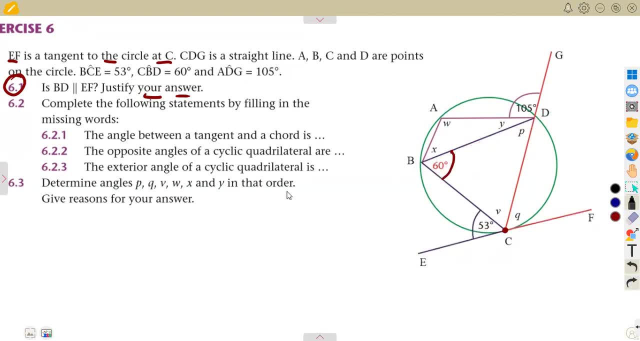 They are not equal. So meaning to say this here is not All right, So not that's. if you were to consider, if we were to have alternate angles, if we were to create a Z, we were supposed to have equal angles, but these ones, they are not. 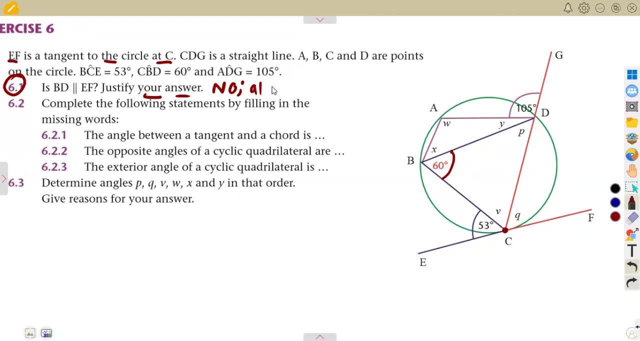 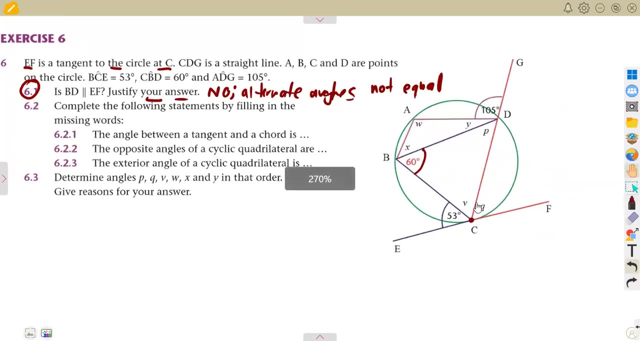 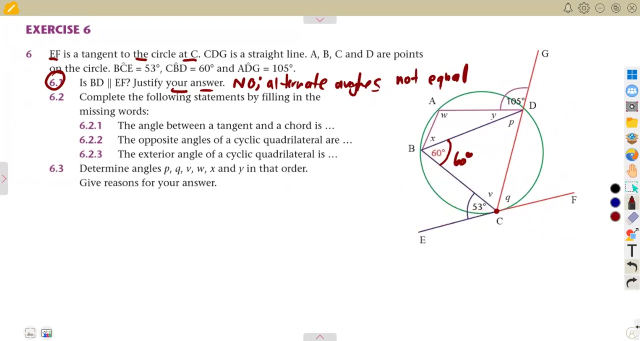 So alternate angles not equal on this one, All right. Alternate angles not equal or unequal, So they were supposed to be equal. If truly they are parallel. we are going to see that this was supposed to be 60. This was also supposed to be 60. So that we talk of what Alternate angles? But in this case they are not. 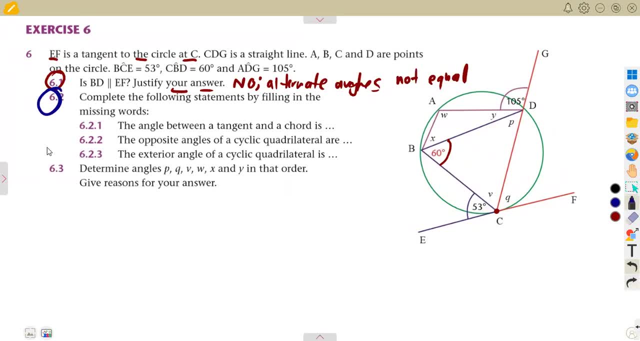 So meaning to say these two lines are not Complete the following statements: So in this case, you are supposed to answer this by filling in what is missing on these statements. The angle between a tangent and a chord is. They just ended there. 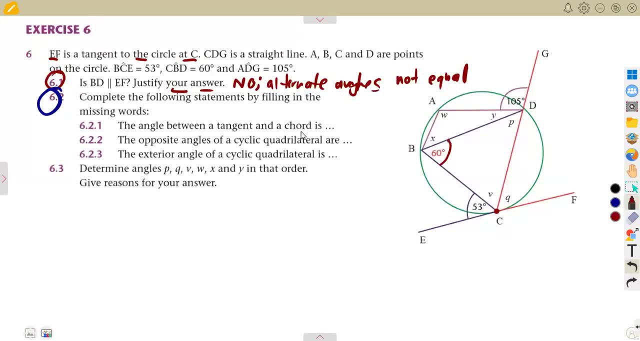 They just ended there- The angle between a tangent and a chord. So this is a theorem. Remember that the angle between a tangent and a chord is equal to the angle in the alternate segment or in the opposite segment. So that one, the angle, there's going to be 6.21.. So this one, it is equal to the angle. 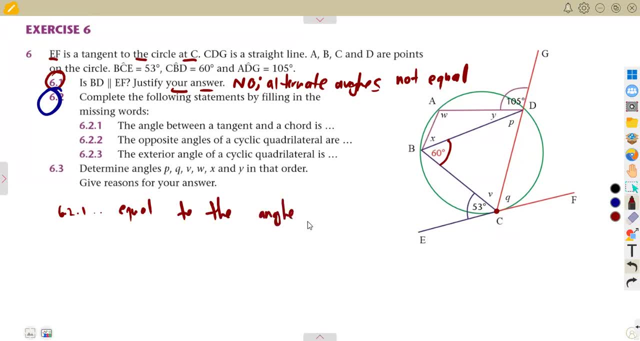 Subtendence Subtended, All right. So it's going to be equal to the angle subtended, to the angle subtended. So the angle is going to be subtended by the chord, All right By the chord, But when subtended by the chord, where In the alternate segment, 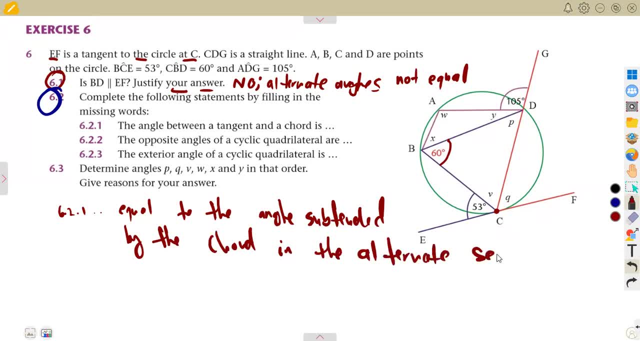 In the alternate segment All right. So that is the idea there. So the alternate segment means All right. The hole. Kelsey here says it's equal to the angle subtended by the chord. So that's what you're measuring. You've got the angle subtended by the chord. 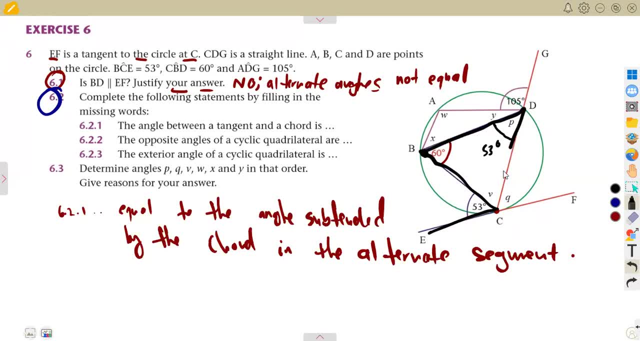 All right. So what you're measuring when you continue to just say we're going to do just this one? what's the angle subtended by the chord? Well, if the greyguru would just say: well, that is equal to the angle subtended by, currently determined by this result here, which means we can make this clear. 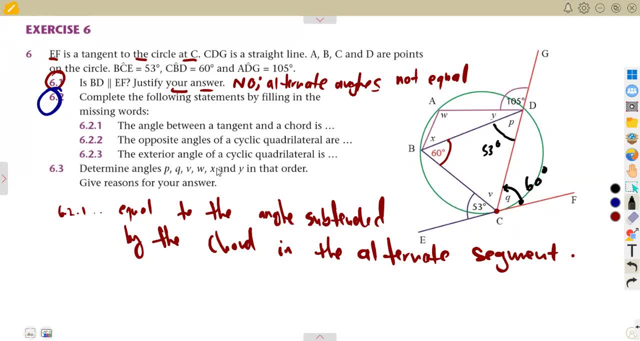 Of course you can go at. I said it was equal to the angle subtended by this result here, Right, And the Pennsylvanian opens this here. All right, So we go ahead And it's equal to at office. 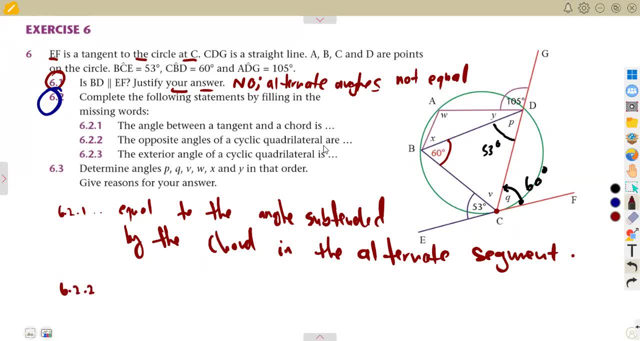 what this is all about: the opposite angles of a cyclic quadrilateral. opposite angles. if you're given a cyclic quadrilateral, you know that opposite angles are supplementary, they add up to 180. so these ones, they are supplementary, they add up to 180 degrees. all right, another part that you're 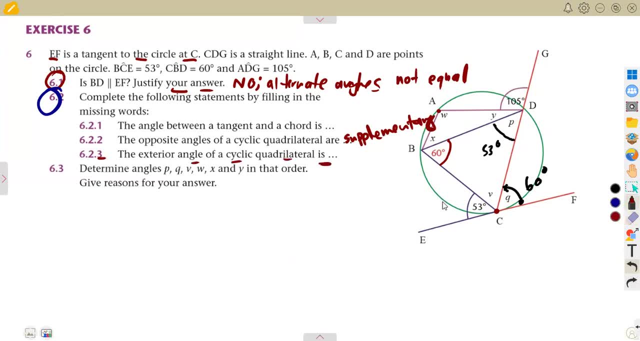 given the exterior angle of a cyclic quadrilateral is the exterior angle of a cyclic quadrilateral is equal to the opposite interior or the interior opposite- I don't know the way that you're going to take there- so this one is equal. they are equal all right to the interior. 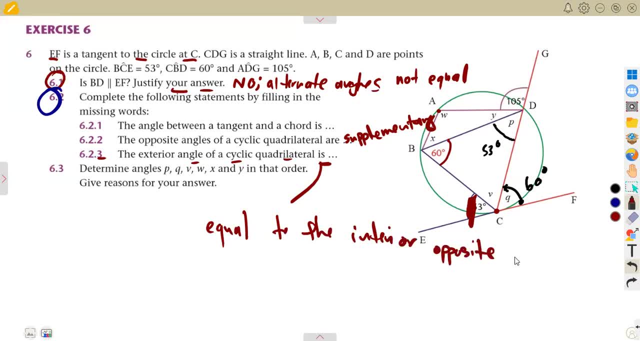 opposite angle to the interior opposite angle or the opposite interior angle. that's the idea of a cyclic quad, all right, and the exterior equality of a cyclic quadrilateral is the exterior McLaren right, the interior McLaren angle there, all right. so the other part there was to determine angles p, whatever that you have in. 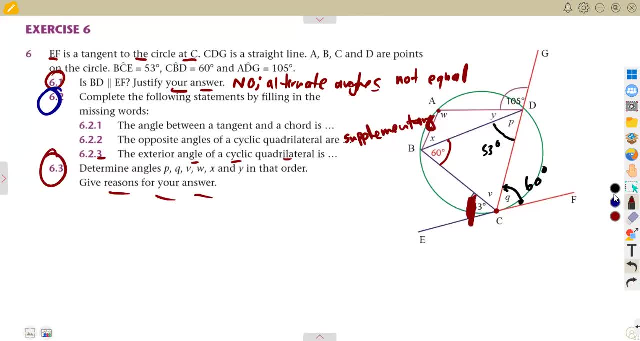 that order. give reasons for your answers. all right, so in that order. all right. so let's see p? uh. already we said p is um going to be 53 degrees. all right, so p 53 uh degrees. the reason, uh, that is the tan chord. all right angle between a tangent and a chord. so i'm just going to write in short. 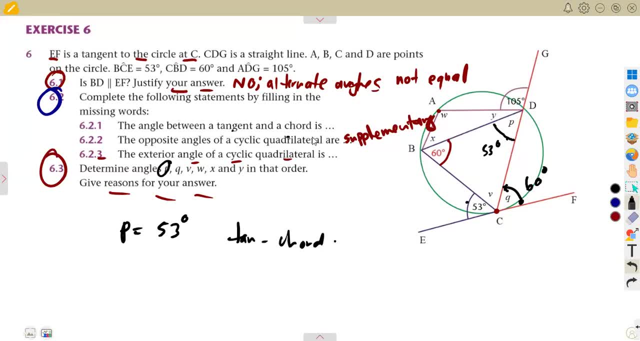 uh, tan chord, but this is the one that we talked about, the angle between a tangent and a chord. all right, then we move on to angle q. angle q also talked about these 60 degrees from the same theorem. uh, we saw that this is 60, so this is gonna be 60 degrees also, all right. angle v, angle v. 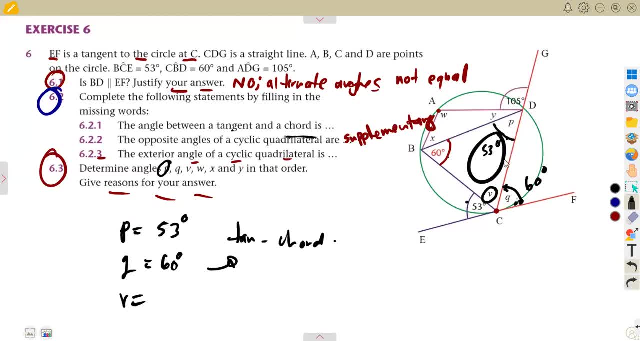 considering angles on a straight line or considering angles in a triangle, it's up to you. so it's gonna be 180 degrees. you subtract. if you're using angles on a straight line, there is a 53 degrees. on the straight line, there is also a 60 degrees. 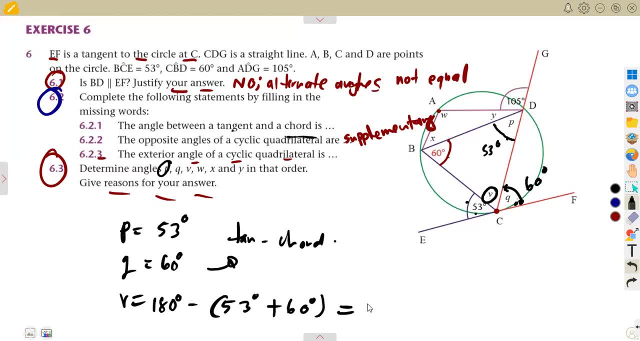 you subtract if you're using angles on a straight line, there is a 53 degrees on the straight line on the straight line, so you're going to subtract all these angles that we are seeing from 180 and that was going to give us 67 degrees. so you can consider angles on a straight line. you can consider. 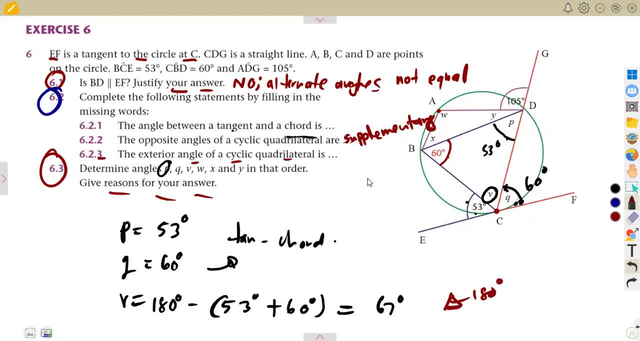 angles in a triangle equals to at 180 degrees. all right, that's our angle b, then angle w, which is this one. considering a, b, c, d, this is a cyclic quadrilateral. all these four points are on the circumference of a circle. so we said the opposite angles of a cyclic quadrilateral are supplementary. 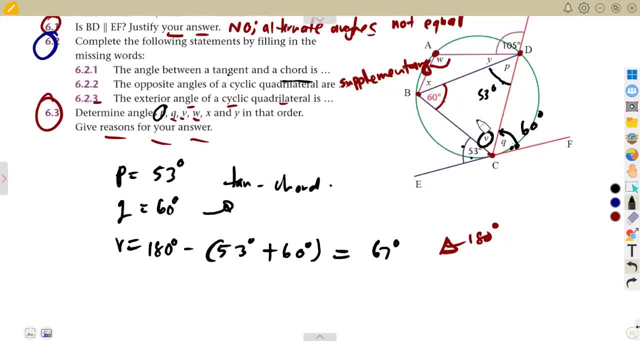 they add up to 180 degrees. so meaning to say, if this is 67 degrees, our angle w is going to be 180 degrees minus 60, minus 67, uh, degrees. that was the, that was the condition, and this was going to be 113 degrees. so there we are simply talking about. 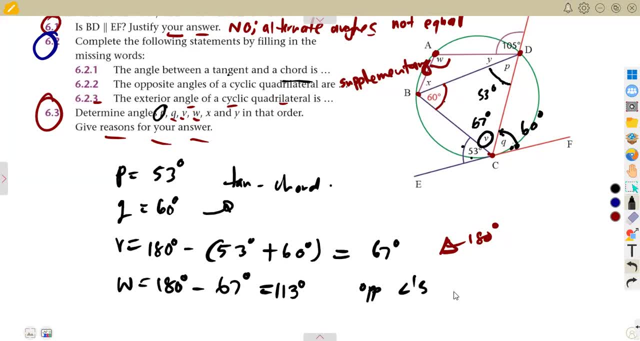 opposite angles of a cyclic quad, opposite angles of a cyclic- uh quadrilateral. so they are supplementary. all right, so that means this was going to be 113 degrees, all right, angle x. how can we determine angle at x? all right, so there were so many ways? uh, actually not so many ways, but uh, you can use. 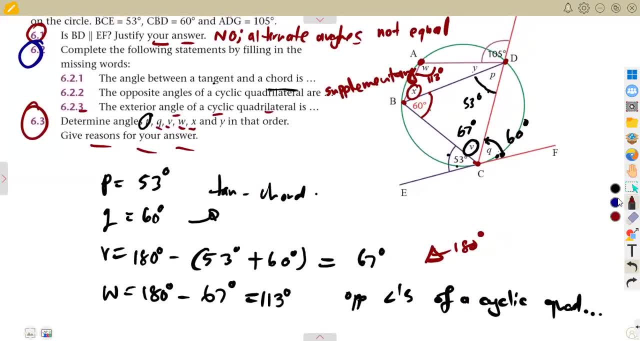 this concept here. uh, angle x is going to be 113 degrees. all right, so this was going to be 113 degrees. so here we are, counting our Square Run here and these two areas will- and if you count them, b zz into square run and thisánhода with exactly the same angle. 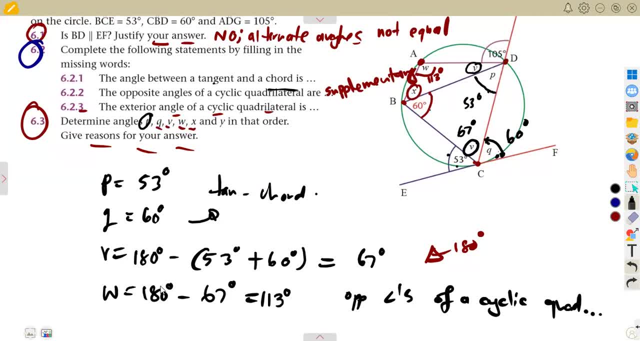 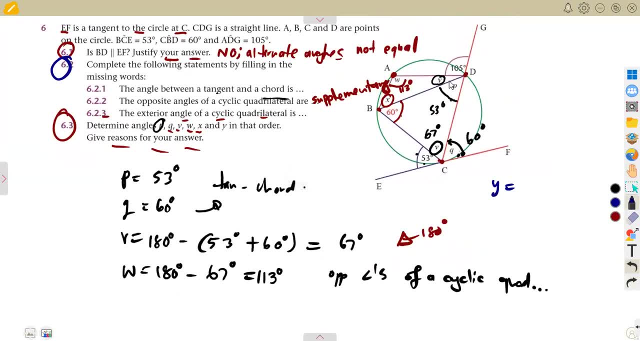 that's going to be Eıyoruz cabinets, minussecretor, at square run and absolutely this angle is equal to the posts of the square run of the course, or this angle, because we could say these angles are angles with a straight line and these angles are angles on a straight line, or this angle is going to be the same as the corner. which we just calculated, that is, there, is not fully actually proportional to that. now, according to this anglO itself, with respect to the angle at large and xz, there is two angles that are angles on a straight line. so there is little bit of difference between angle Because 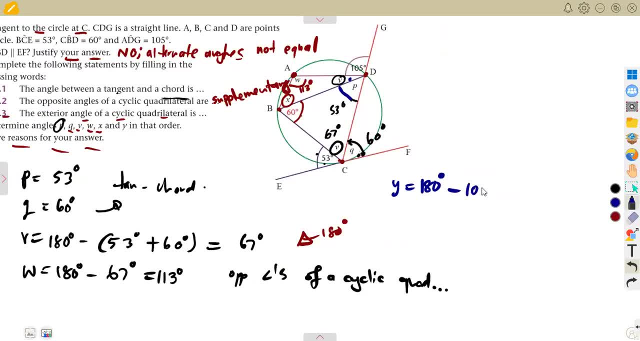 there is two angles on a straight line and it's going to be 180 degrees, that the result is this angle. okay, it also means that you can estimate the angle M from this angle, because the angle M and angle on a straight line there is 105. also there is 53 degrees. you subtract these two or just open. 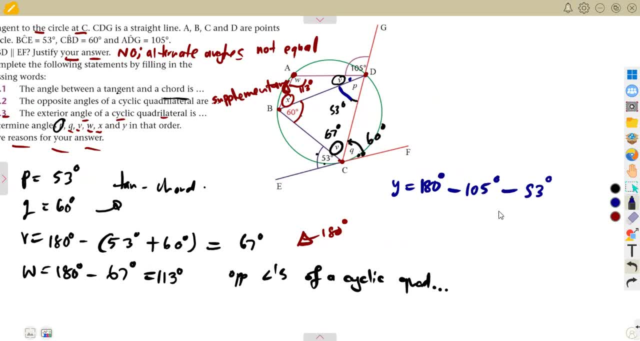 a bracket. then if you open a bracket like this, you add: but if you don't open a bracket, you just minus, minus and so on. so if you were to subtract this, meaning to say we're going to have something like 22 degrees, so this angle y, there is 22 degrees, so it means from there you can determine. 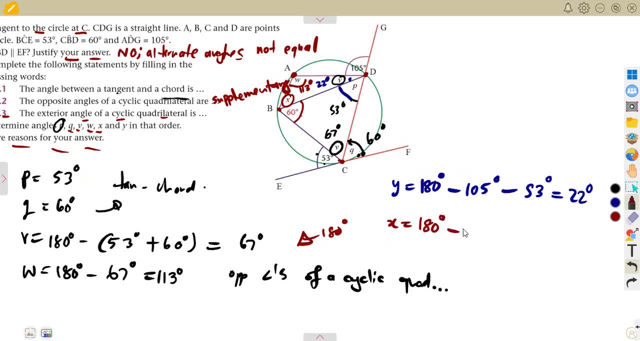 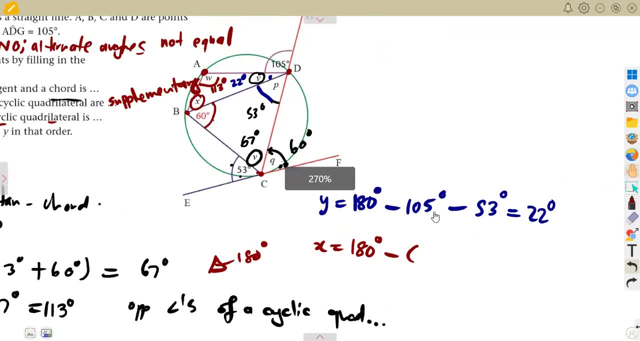 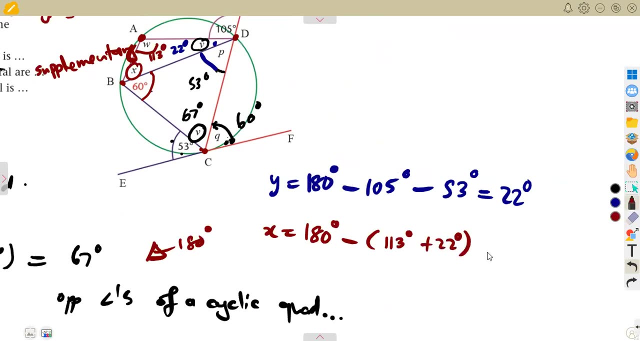 angle, x, angles in a triangle. they add up to 180, so it is going to be 180 minus. like i said, if you open a bracket, you add these two angles, uh, that is the 113. inside of the triangle there is 113 degrees, there is also 22 degrees, so if you're to subtract this, you're going to obtain, uh, 45 degrees at the 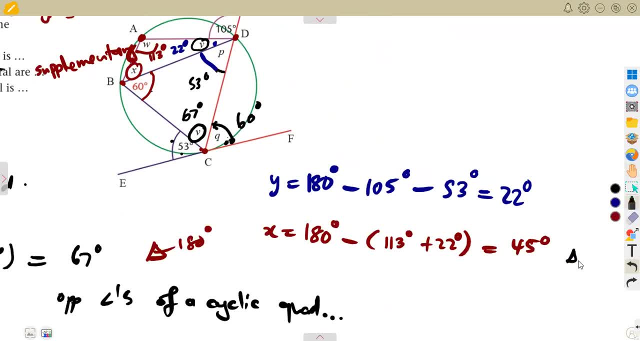 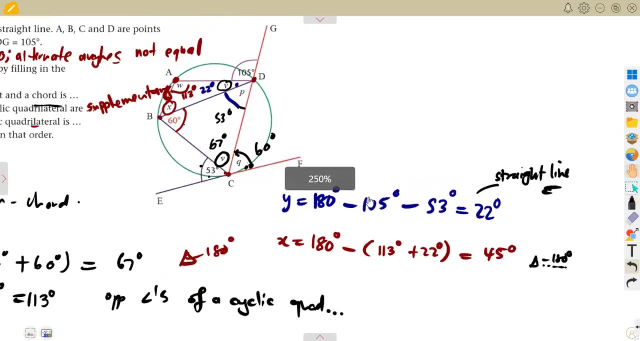 end. so this one, we are talking about angles in a triangle. all right angles in a triangle add up to 180. this one we consider angles on a straight line. this is about angles on a straight line, angles on a straight line. so this is how you can attempt these typical questions. what you need is to make sure that 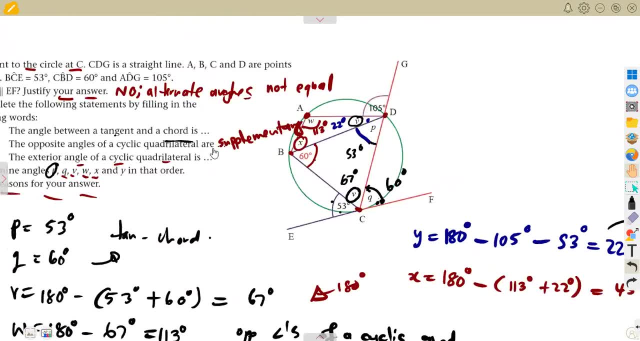 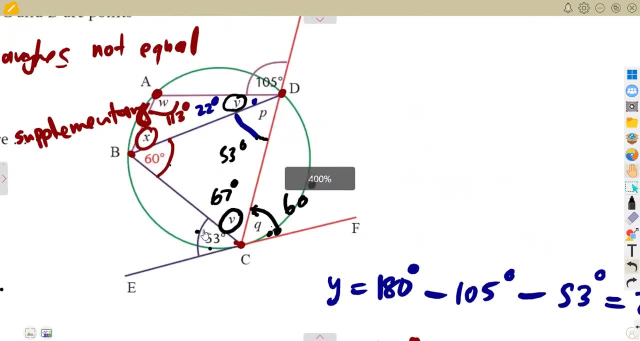 you have your theorems and work with your theorems together, you can answer any typical question that you might be given in your examinations. in your final examinations, let's revise as much as we can.